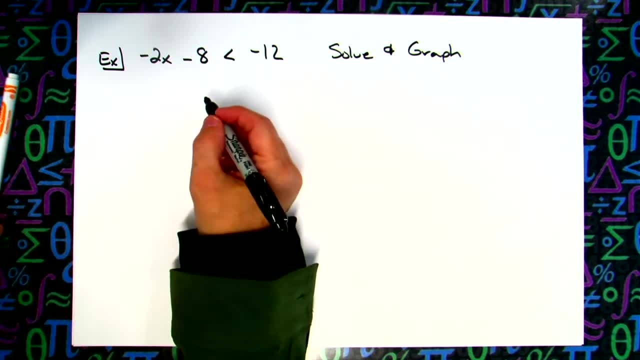 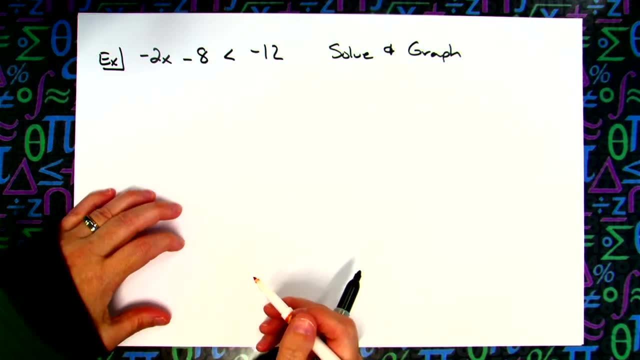 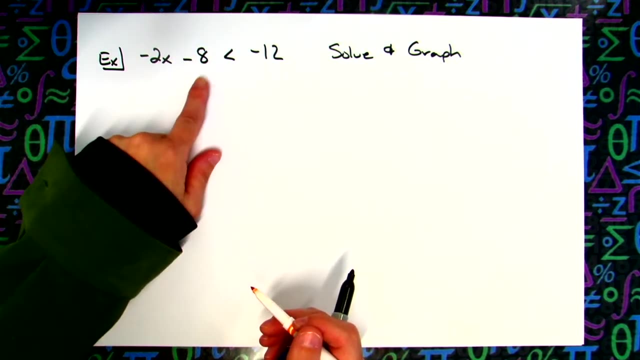 on there, since that was kind of new. All right, so on this, this is a two-step equation, Clayton. what's the first thing I'm going to do to both sides? I don't want to divide. I'm going to divide first because this is a two-step equation. So when I do a two-step, 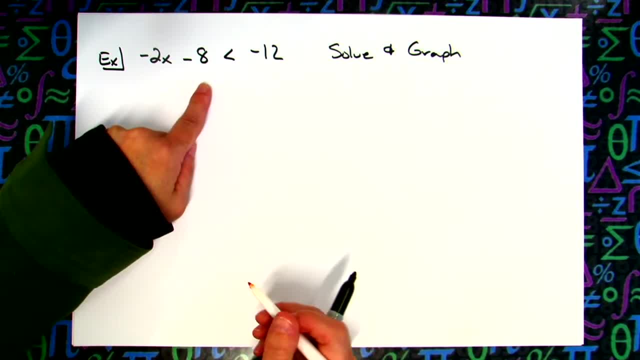 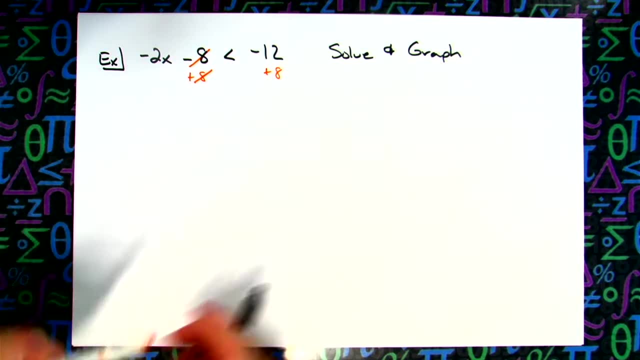 equation, I always have to add or subtract first. So I'm going to add 8 to both sides. So I'm going to add 8 there. I'm going to add 8 right there. Okay, this works just like a two-step equation, So that negative 2x comes down and the only difference is, instead of having an, 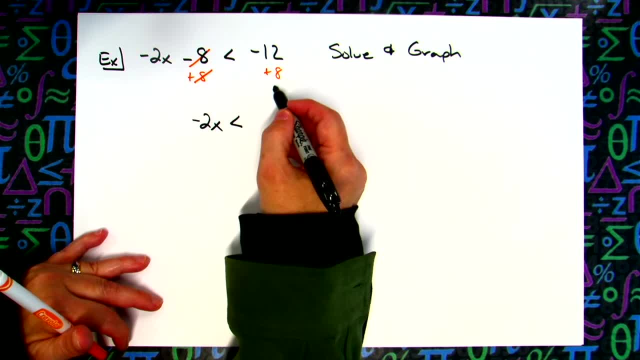 equal sign. I have a less than sign. All right, then I'm going to do this over here. Negative 12 and 8 is going to give me a negative 4.. Okay, Griffin, what am I going to do now? 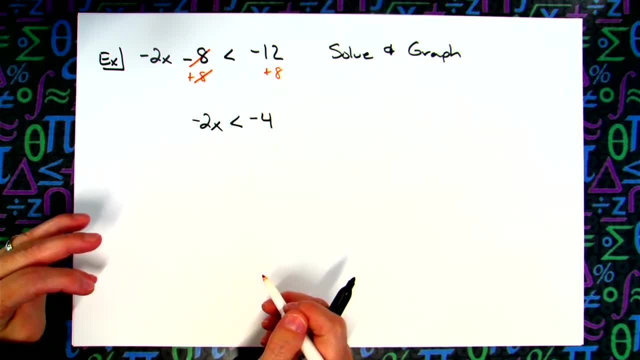 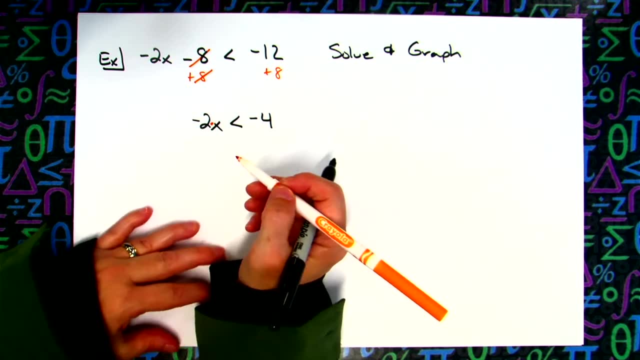 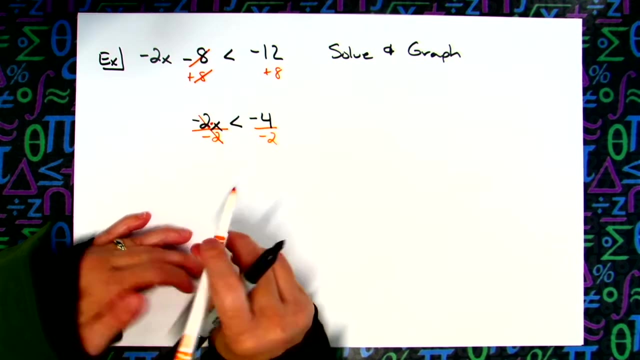 I'm not going to multiply them together, because this is negative 2 times x, What's the opposite of multiplying Division. So I'm going to divide by a negative 2 and divide by a negative 2.. All right, now do I need to flip the inequality? Braden Yep got to flip the inequality, So I'm 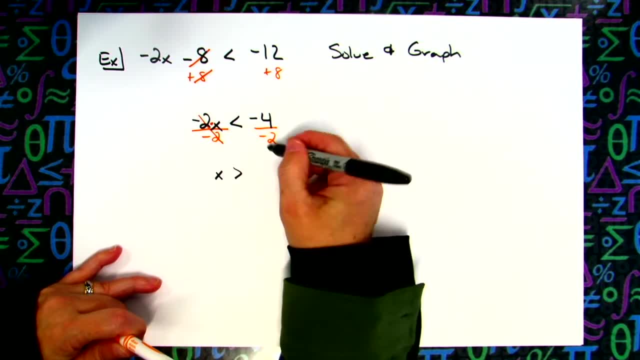 going to go ahead and write the x down. I'm going to go ahead and flip it All right. dividing like signs, It's going to be a positive. I'm going to go ahead and write the x down. I'm going to go. 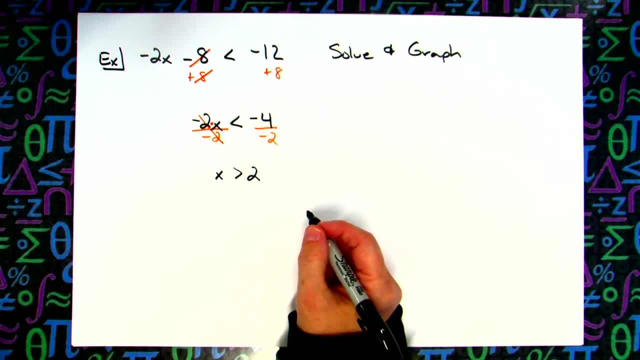 ahead and write the negative 2.. All right, you have to be able to get that part right before you can get the graph right. All right, it's solve the equation and then graph it. All right, now we are going to graph it with an open dot and with our square and curvy brackets. All right, 2 is a pretty. 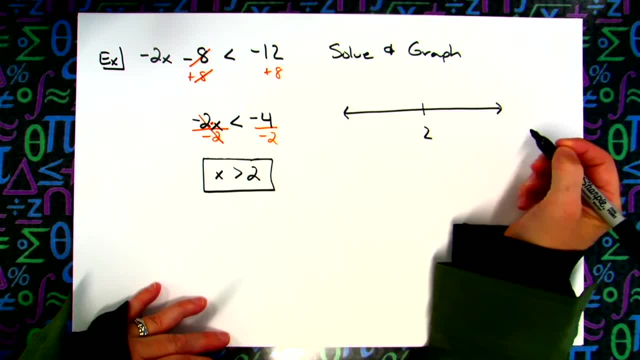 small number. I would still put 2 in the middle of my number line if I was going to do it. All right, I would put a 3 on the right-hand side. I would put a 1 on the left-hand side. Okay, open or close. 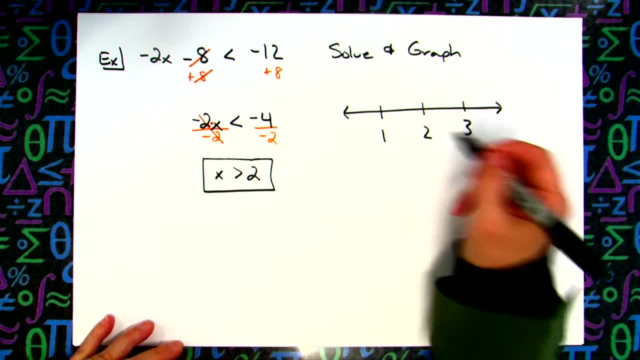 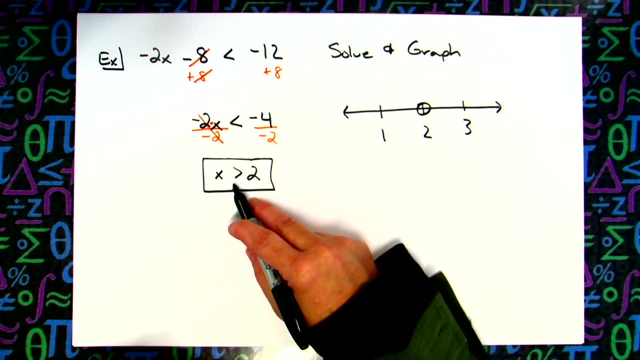 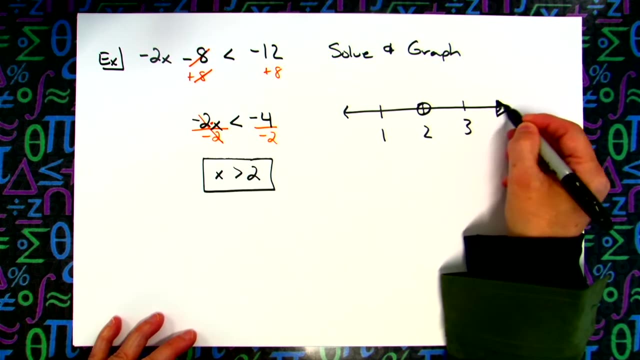 dot. Great open or close dot. Open, Open, dot. Okay, open dot on 2 because of the greater than sign. All right, which way am I going to shade Dallas? which way am I shading Right To the right? Okay, so then we shade to. 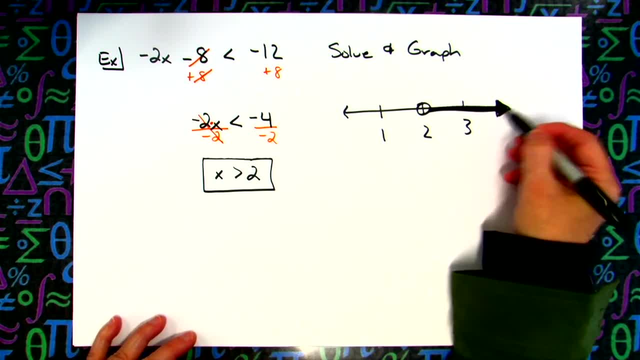 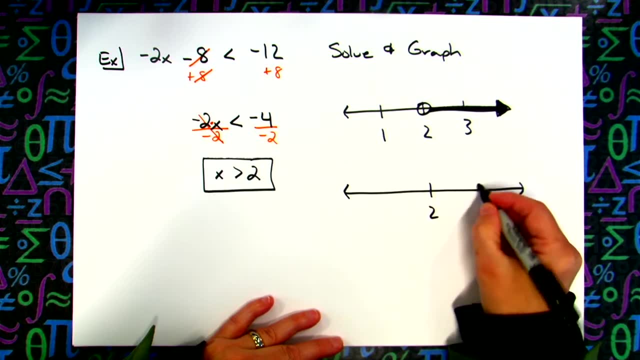 the right And that's what it looked like. And that's what it looked like on the 12 questions that we had done at the beginning of class. All right, but two days ago I also showed you another way, kind of leaning towards that interval notation. All right, 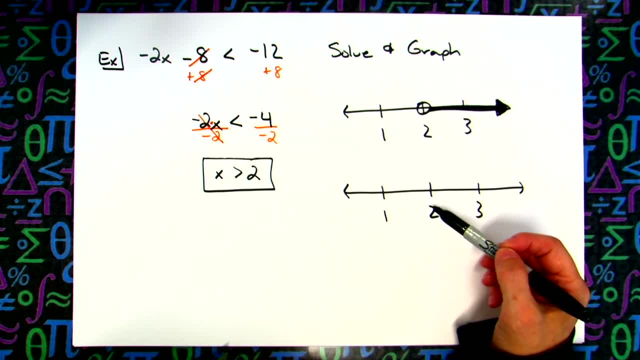 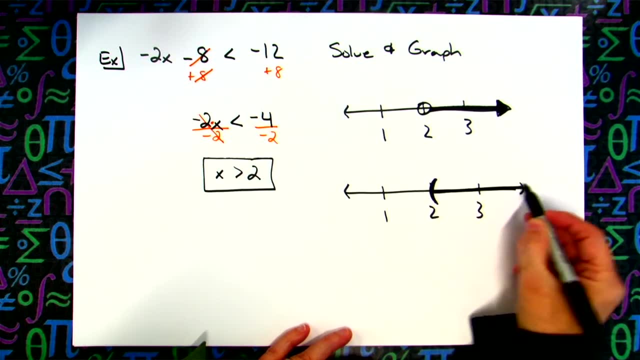 when it was an open dot. we could also use a curvy bracket, And I'm going to make the curve go the way I'm going to shade. so curvy bracket going this way. That's the exact same thing, All right. 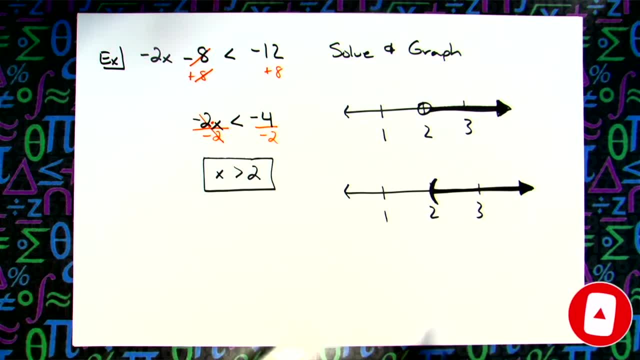 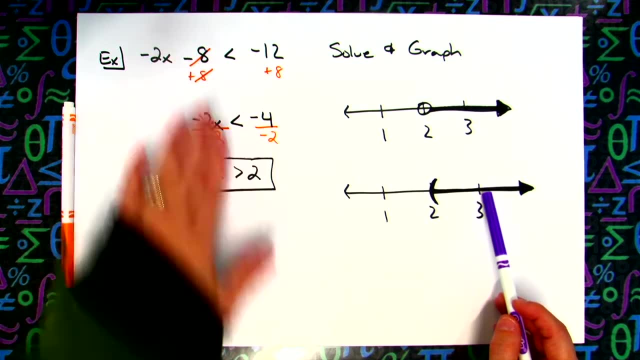 now let's even go one step farther. All right, there is this thing called interval notation. If I can draw something on a number line like this, this is telling me where the answers to this inequality lie. All of these numbers over here make this inequality. 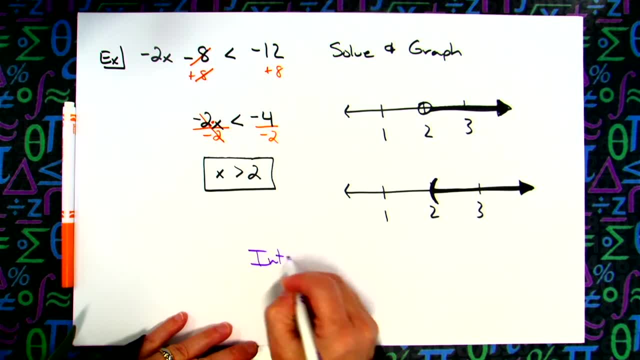 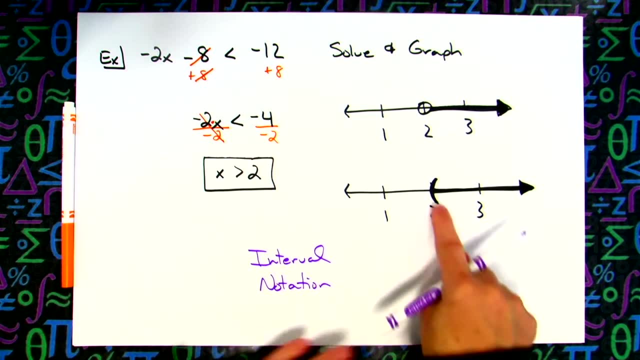 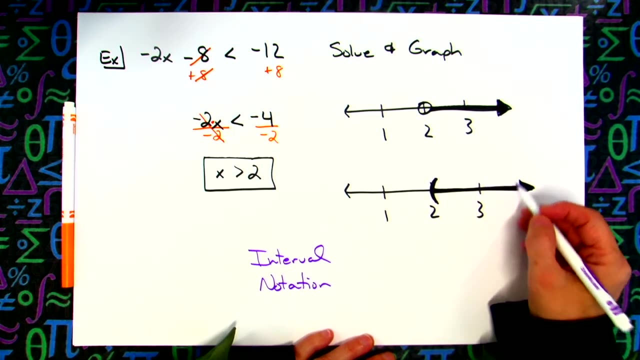 true, All right, so there is something literally called interval notation. I can represent this answer by looking at this number line and knowing that what as I go to the right on a number line- 34567, what? it goes all the way to infinity? right, because the number 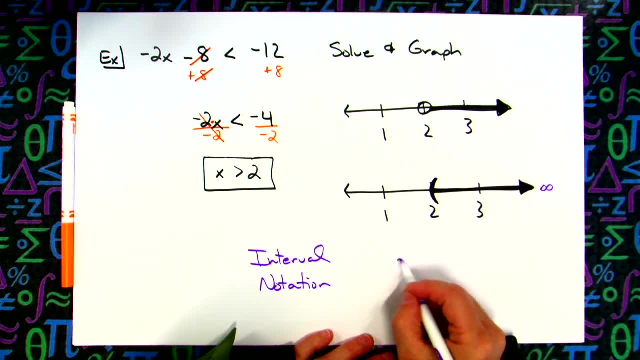 line goes forever and ever and ever and ever. So I can take the two, because that's part of my answer, And I can put the two in the number line. And I can put the two in the number line. And I can put the two in the number line. 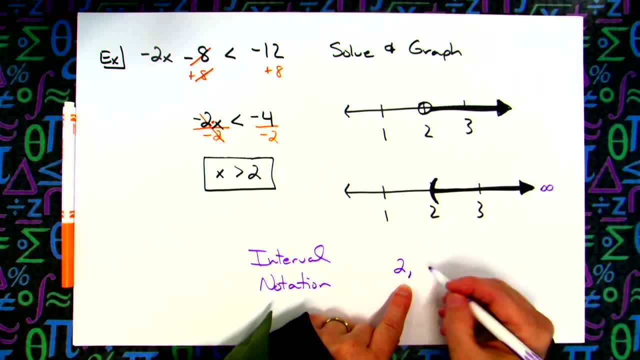 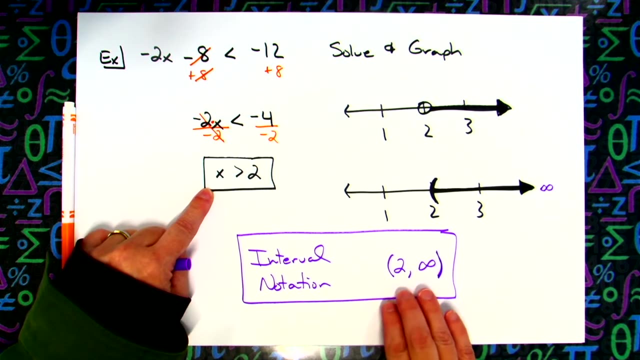 And the infinity, since I've shaded all the way down forever and ever and ever to the right. All right. curvy bracket on two, always a curvy bracket around infinity. So that answer of x is greater than two can also be written in interval notation with two curvy brackets. 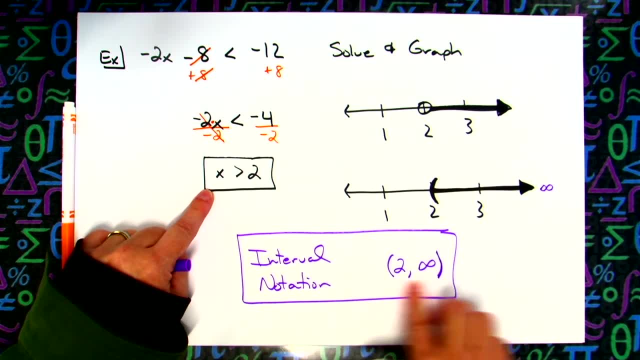 around the two and the infinity. This would be the corresponding number line. This is the corresponding number line there. So everything there is equivalent and the same, And that interval notation is the same. So I can put the two in the number line And I can put the two in the number line. 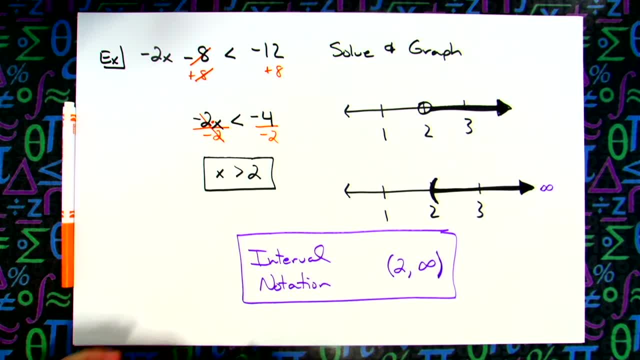 is new. It's what you've not seen. okay, The next time we do questions on the, you know, like the multiple choice questions at the beginning of the class, instead of having the open and closed dots, I will probably have the curvy and square brackets. okay, All right, so let's do another. 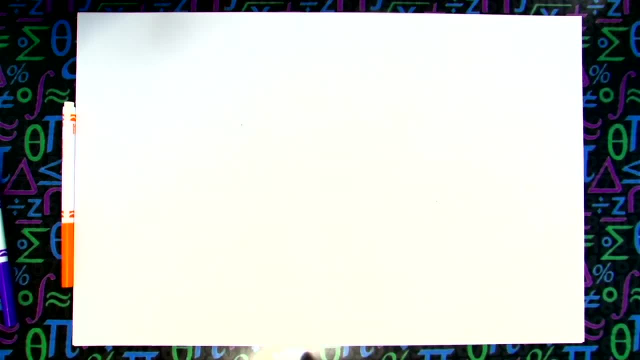 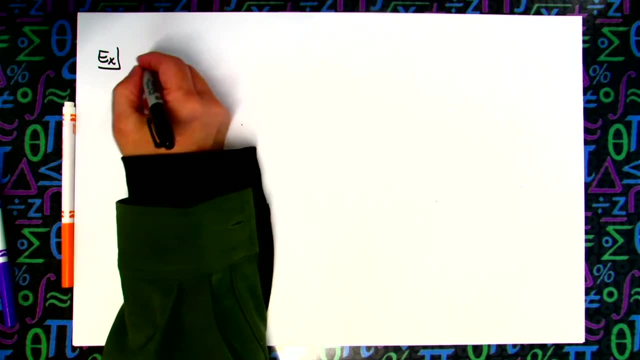 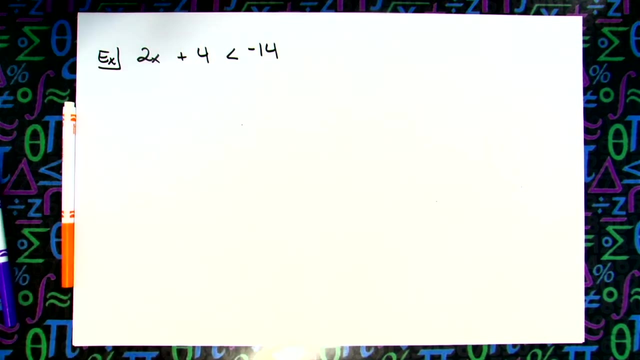 one of these. all right, Pretty much everything in Math Excel is going to be: solve it and then graph it. okay, So we're going to take a look at something like: maybe a 2x plus a 4 is less than a negative 14.. All right, again, it's probably going to tell you to solve and graph. 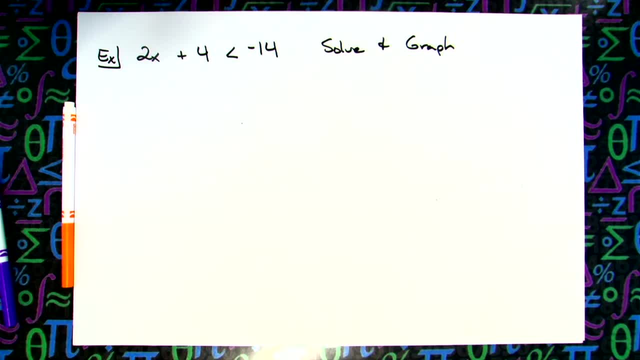 And we're going to do both number lines with open dot, closed dot, curvy and square- Actually, let's make this less than or equal to- And we're also going to do the interval notation. All right, it's a two-step equation, all right, Noah, what am I going to do to both sides first, 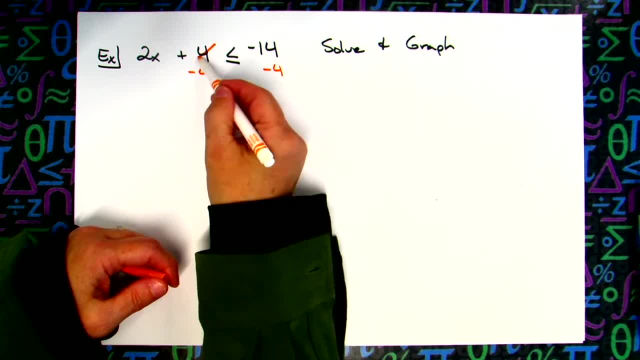 Yep, we're going to subtract 4 and subtract 4.. So the 4s are going to go away. all right, It's going to be just like a two-step equation, except I have the inequality symbol, So the 2x is going. 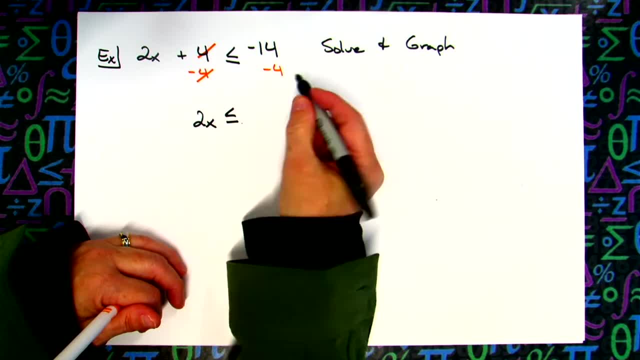 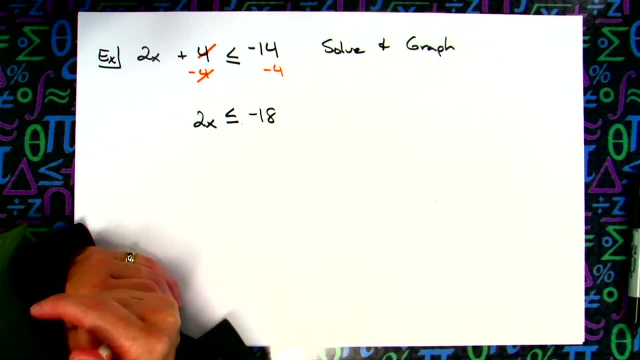 to come down. I'll bring down the less than or equal to Negative 14, and negative 4 is like a negative 18.. All right, I'm going to then do what? to the next step, Abby, what am I going to do in? 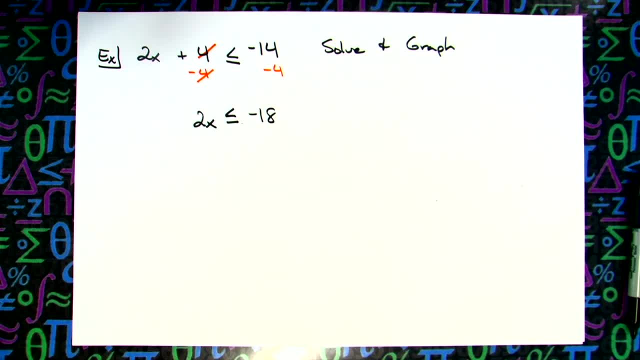 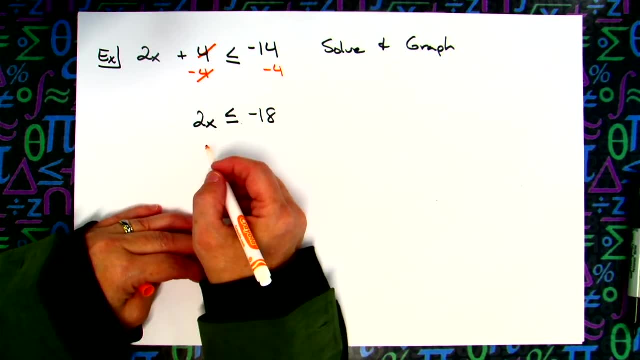 the next step. All right, I don't flip it. All right, am I going to multiply or divide by the 2?? Yep, I'm going to divide by the 2, and I'm not going to flip it because the 2 is positive. So 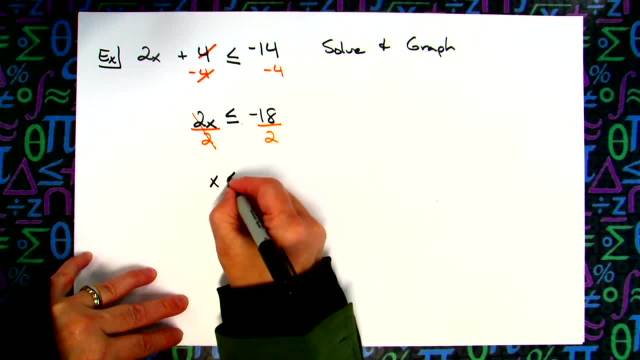 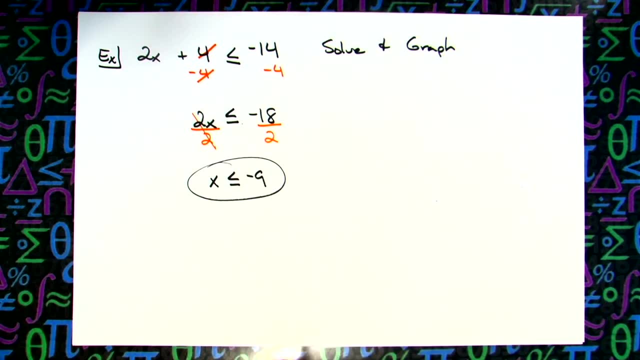 I'm just going to keep that inequality symbol. I'll have: x is less than or equal to, and then when I divide there, I get a negative 9.. All right, so that's an answer, right there. Okay, when I do, I'm going to do my first number line with a negative 10, and then I'm going to do my 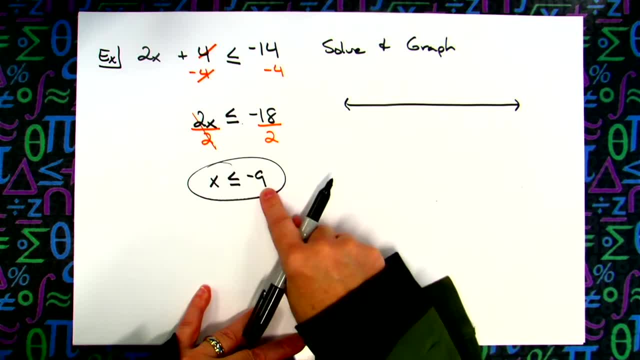 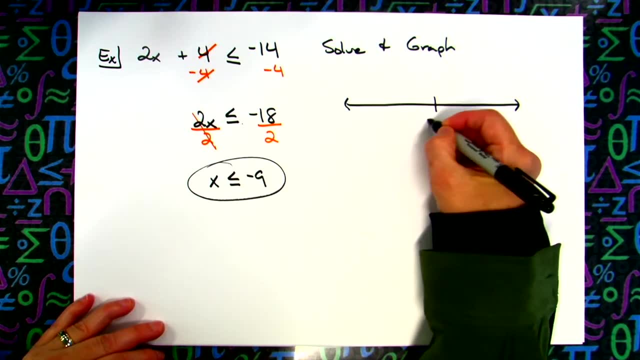 number line with a negative 9.. So I'm going to do my first number line with a negative 10, and then an open dot. whatever number is right there, doesn't matter how big it is or how small it is. always put that number in the middle of your number line. all right, put one number on both sides. okay, so to the 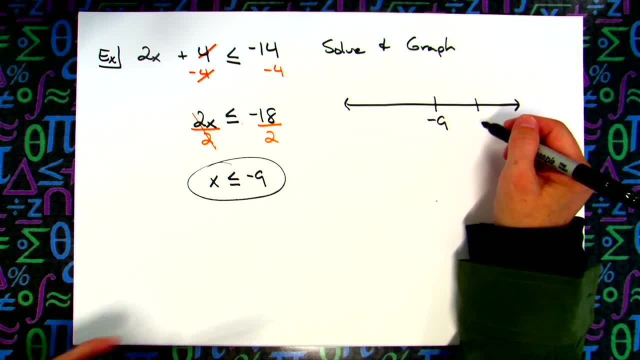 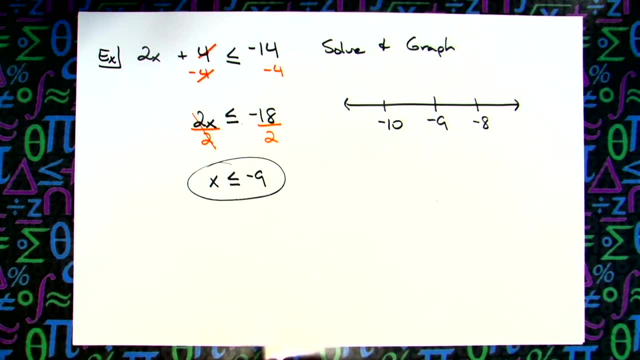 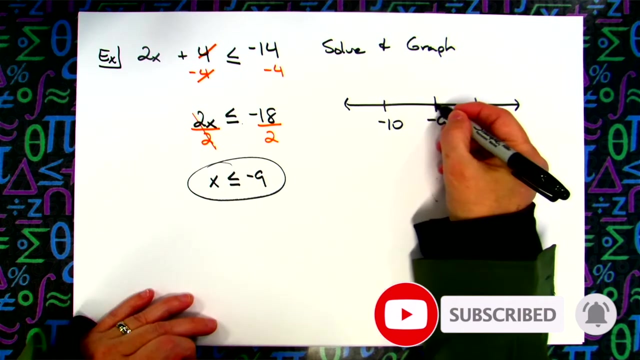 right, what number goes to the right? go the other way. yep, negative 8 over here and negative 10 over here. okay, what kind of dot on the negative 9, Clayton? what kind of dot on the negative 9? I got the equal to part. so closed, yeah, closed. so we're gonna do a closed dot. all right, now, this. 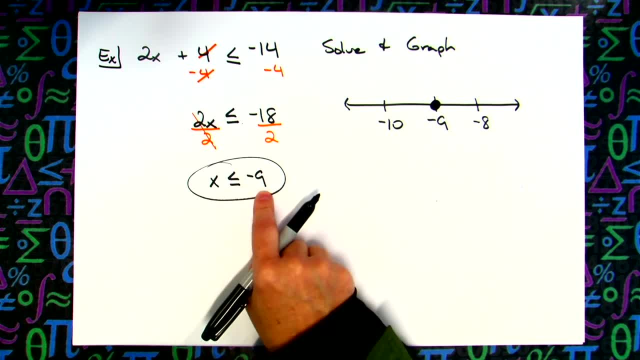 says X is less than or equal to negative: 9. all right rain. which way am I going to shade? am I going to shade to the left or am I going to shade to the right? where are the numbers that are smaller than negative? 9. yeah to the left. 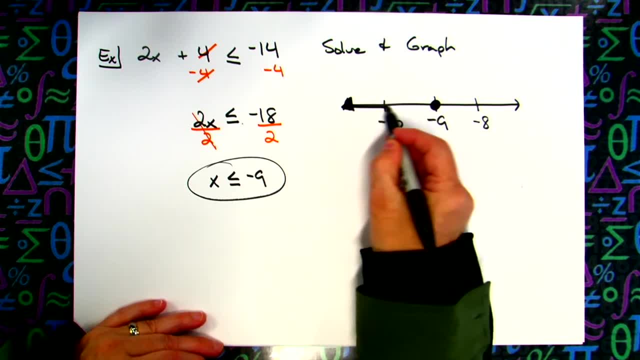 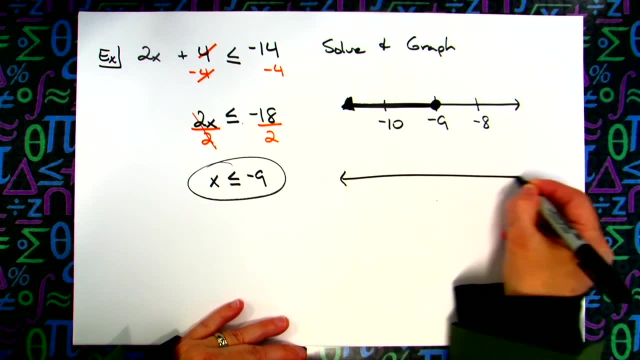 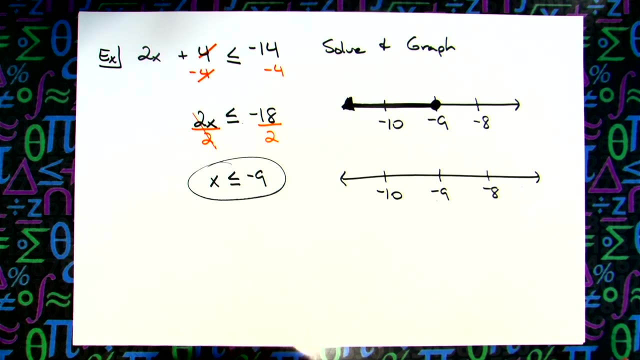 okay, so we're shading to the left. all right, so that's what the number line looks like with open and closed dots. okay, you draw it again. put the numbers in the exact same spot. what kind of bracket do I need on the negative? 9 is gonna be curvy or square. Carter, is it gonna be curvy or? 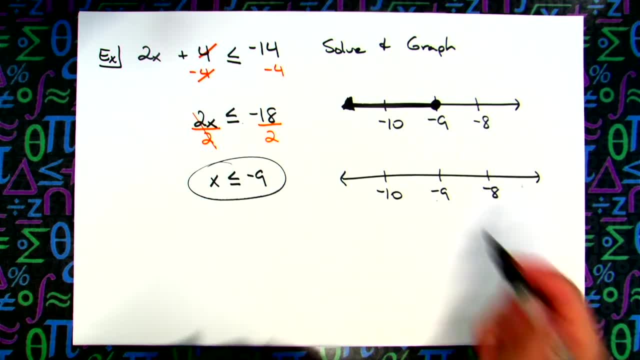 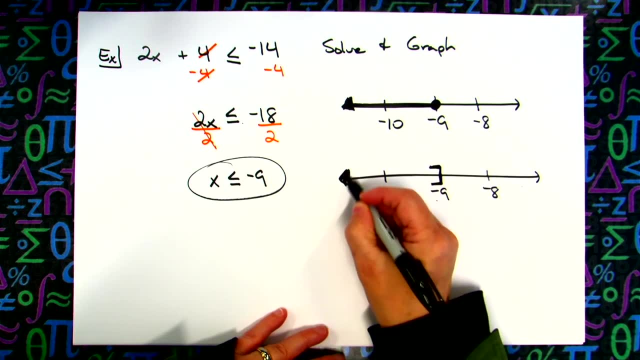 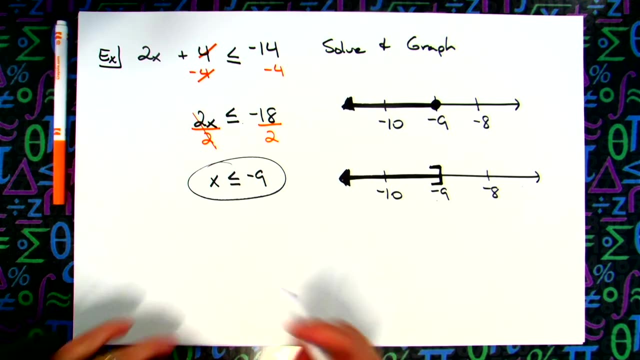 square. it's gonna be square and since I already know I shade to the left, I'm gonna make my square bracket kind of go to the left and then everything gets shaded to the left. all right, then, if I asked you to write the answer in interval notation? all right, now we're gonna look at this number line. we're gonna have a square. 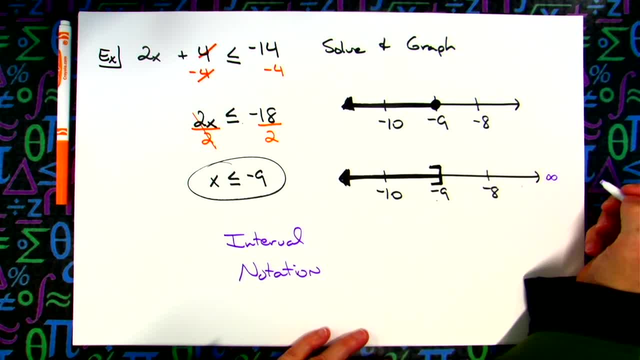 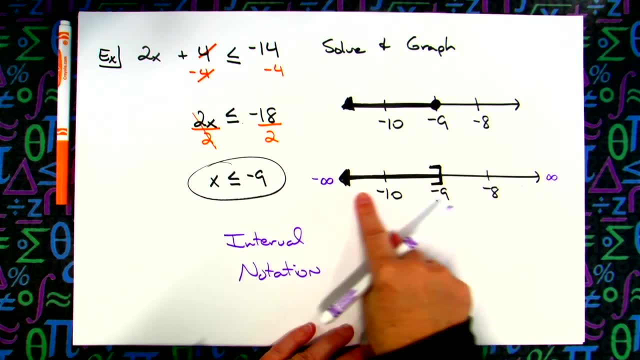 bracket on here. if I have positive infinity down here, what's down here on the left-hand side of the number line, Negative infinity? All right, I am going to look at this number line and I'm going to write the things down left to right. So the first thing I'm going to write down, since I shaded, 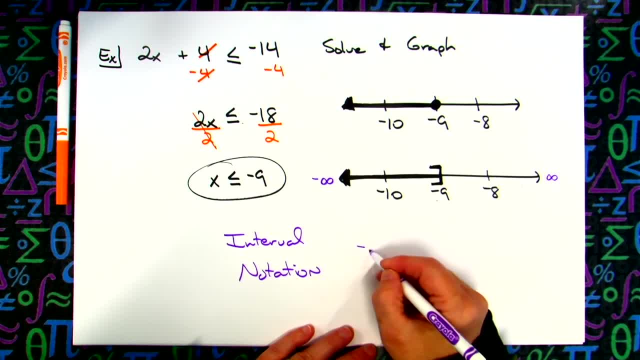 all the way to negative infinity. I'm going to write down negative infinity Infinities always get curvy brackets. always Negative infinity, positive infinity. I always put a curvy bracket by it. All right, then I'm going to put the main 9, the main number negative 9, and I'm going to